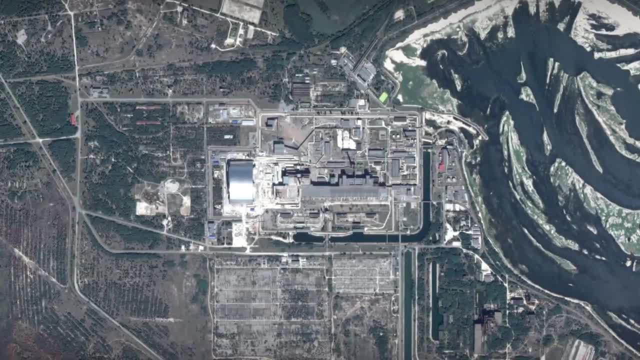 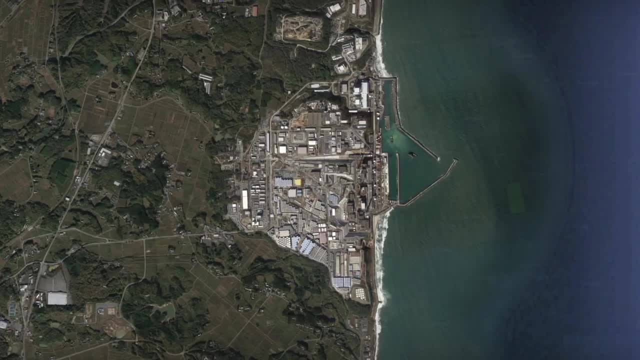 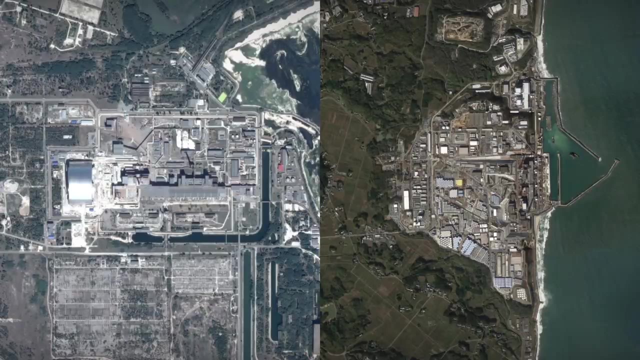 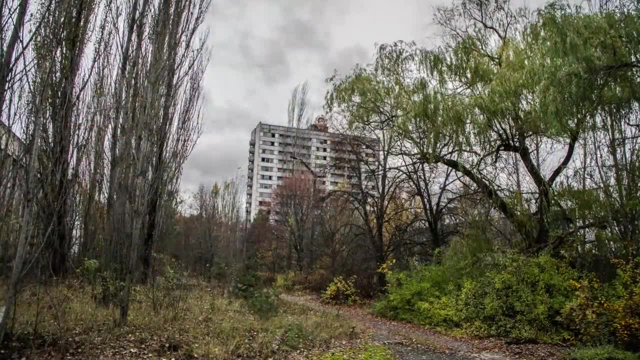 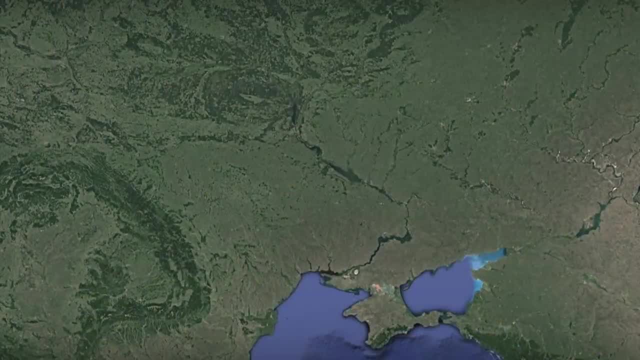 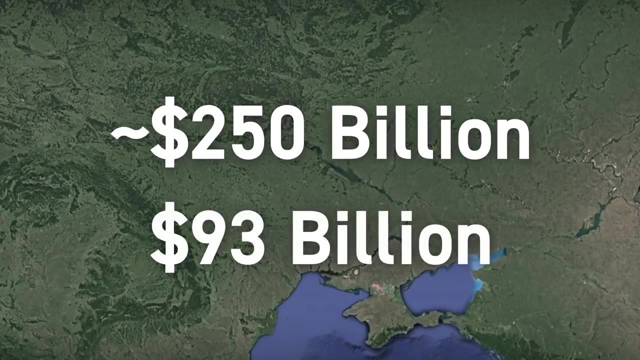 and cannot live due to ongoing radiation. Hundreds of thousands of people were displaced from their homes and will never be allowed to return. The economic damage of Chernobyl is estimated at nearly $250 billion, significantly more than the GDP of Ukraine. The Fukushima 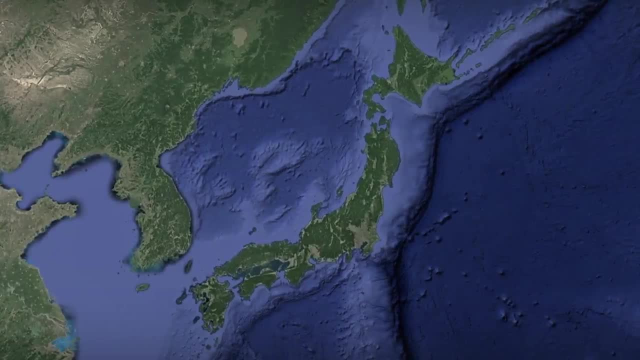 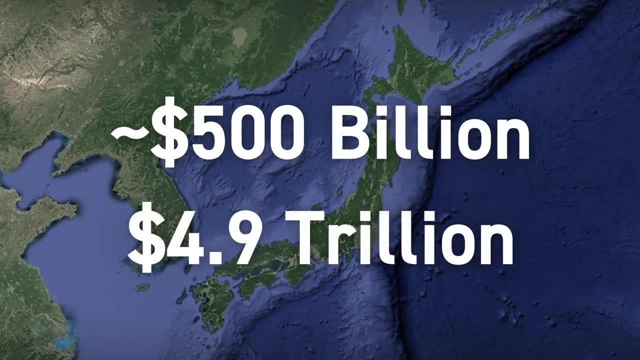 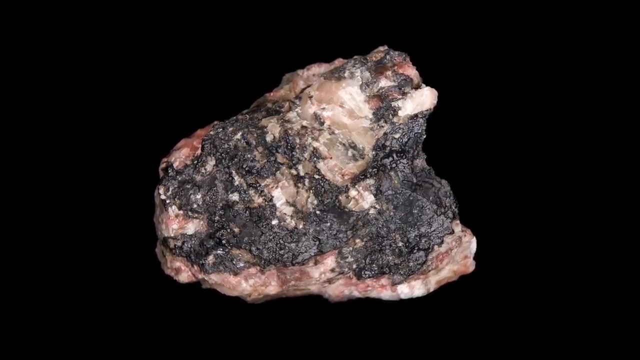 disaster, meanwhile, having taken place in a much more populated and developed area, is expected to set Japan back over $500 billion, a full 10% of their GDP. In addition, uranium, the element most commonly used in nuclear reactors, is not in limitless. 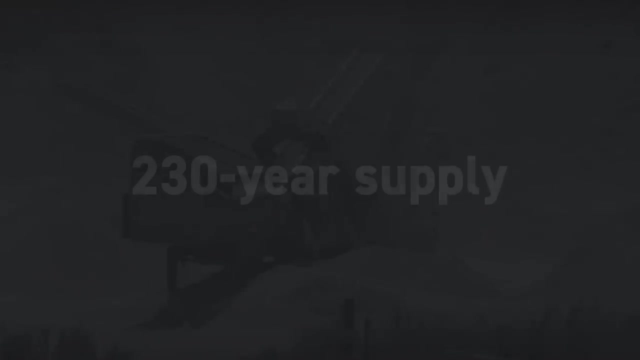 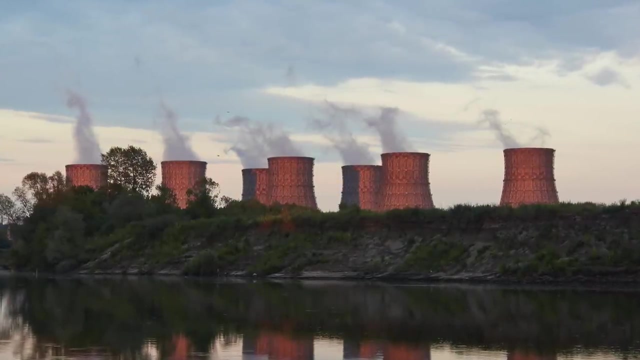 supply. Using present-day extraction methods, there's only about a 230-year supply of uranium left. Many would say nuclear is only a short-term solution to reduce carbon emissions until truly sustainable energy can become commonplace. But the biggest problem with nuclear energy is not the 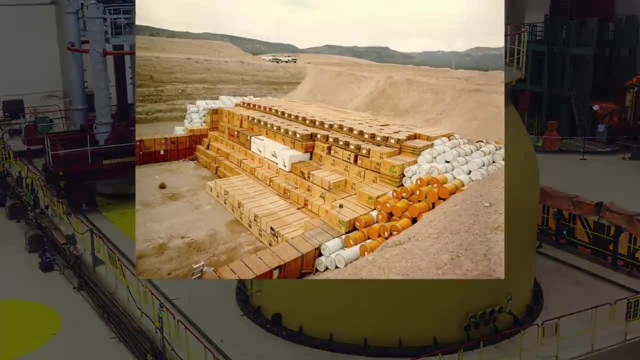 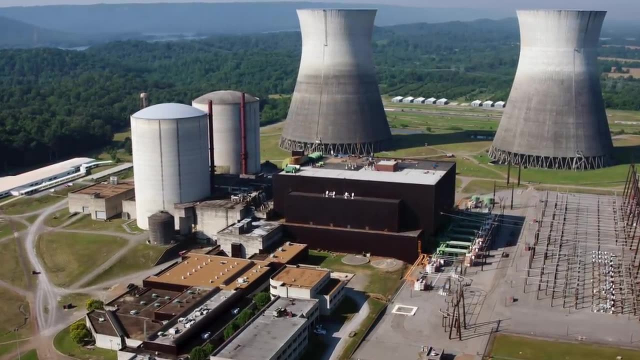 risk of meltdown. it's not the supply of uranium, it's this—nuclear waste. All current commercial nuclear power plants are in a state of emergency. They're in a state of emergency because they're in the process of nuclear fission. As a radioactive element decays, the individual atoms split. 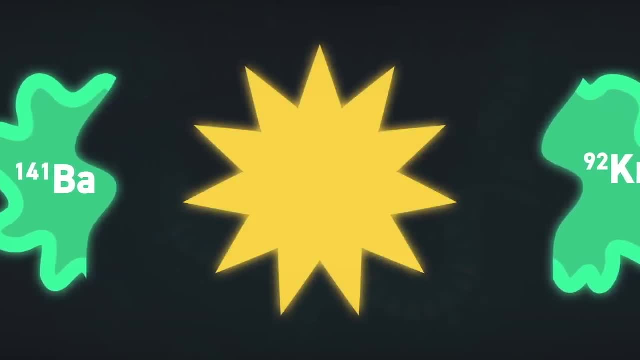 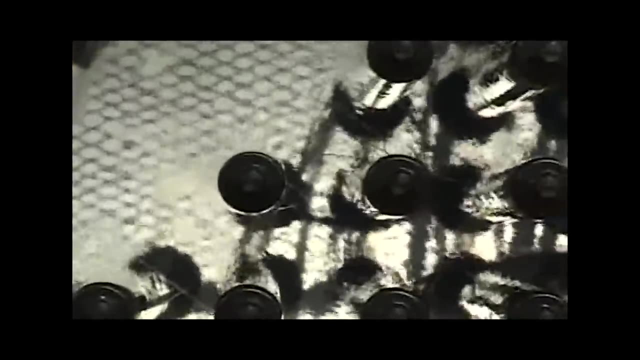 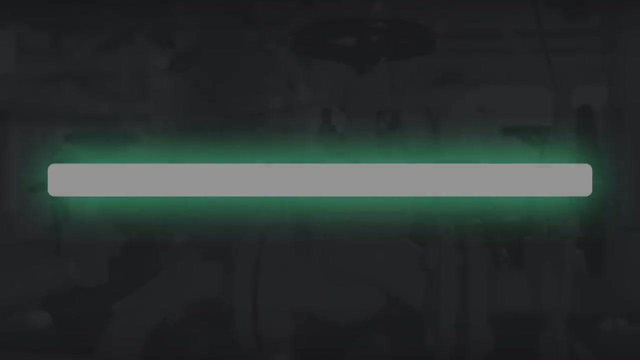 into two, but when that happens, the reaction also releases energy. There are plenty of different designs of nuclear reactors, but in general they capture the released energy by using it to heat up water into steam which runs through turbines that spin generators. The nuclear element used is typically uranium, which, after about six to eight years of usage. in a nuclear power plant will have released enough of its energy that it's likely to be no longer useful in nuclear reactors, but that doesn't mean it's done emitting energy. The fuel rods will remain radioactive enough to emit a lethal dose for tens or hundreds. 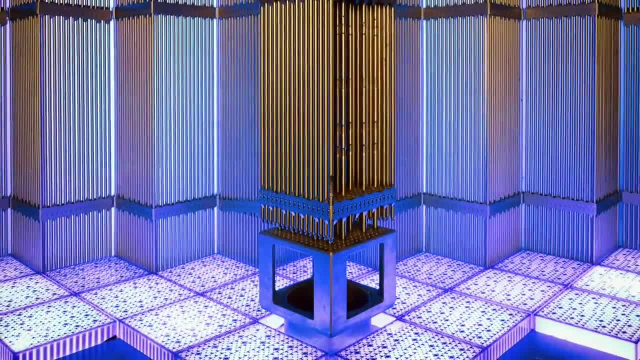 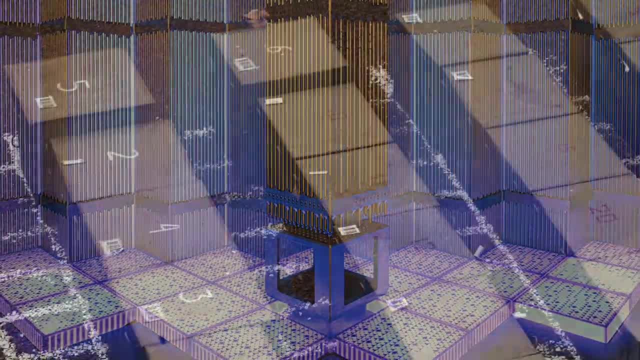 of thousands of years past their removal. So the question is: what do you do with them? The answer is simple: put them somewhere where they can stay undisturbed, isolated, forever. But that's not all that easy. In fact, no nuclear waste worldwide is currently. in what 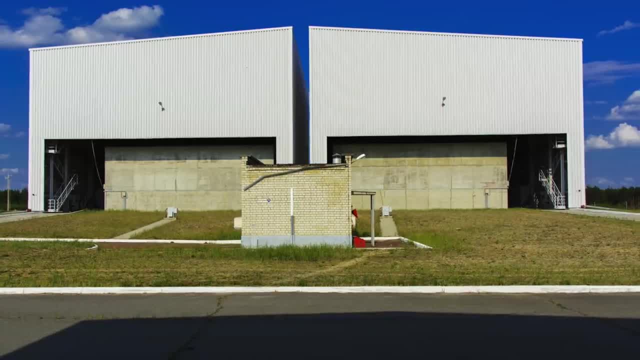 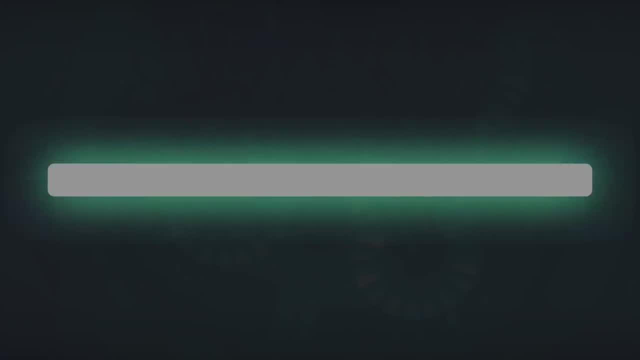 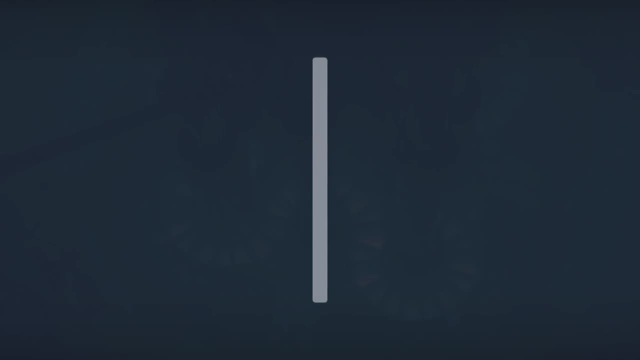 is considered long-term storage. Every bit of nuclear waste in existence is in temporary storage facilities to be used until a long-term solution is built. Most of that nuclear waste is stored in pools of water. Water does a decently good job of shielding radiation, so this is an inexpensive and easy. 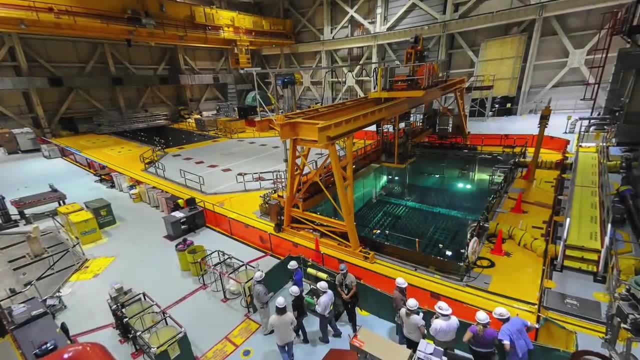 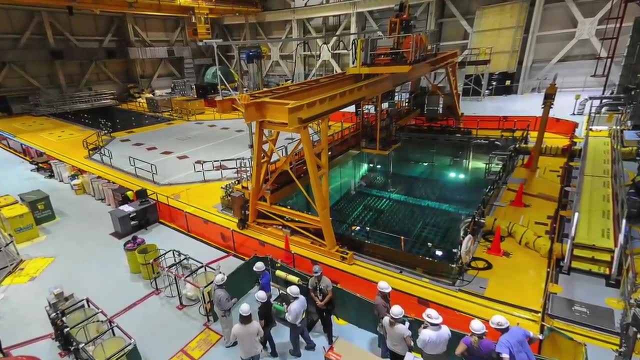 way of storing the rods. Usually, these pools are physically inside the nuclear power plants, so when spent fuel is removed from the reactor, it's put directly into the water and left there. The radioactive material, since it's still emitting energy, continues to heat up the water. but cooling systems and pumps keep the water below boiling temperature. but to do that the plant needs power. If the power fails and the backup generators fail, the pumps and cooling systems stop working. so the water heats up and can boil off The water. 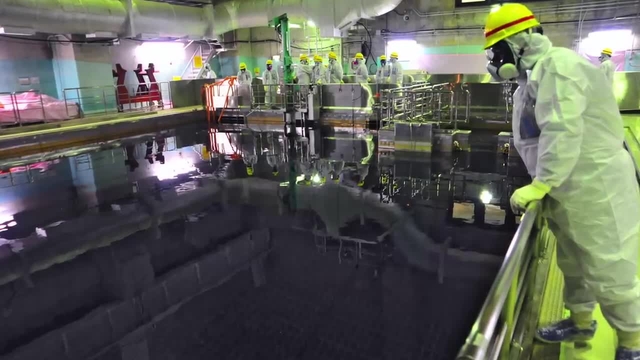 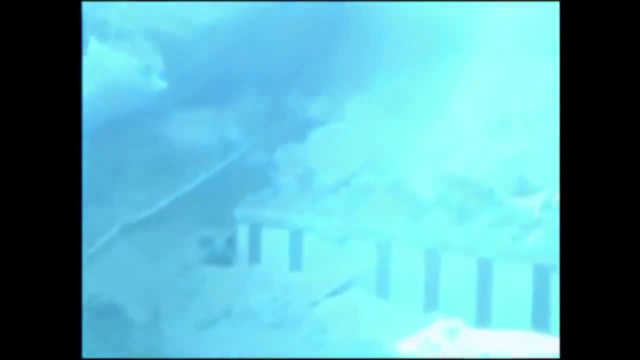 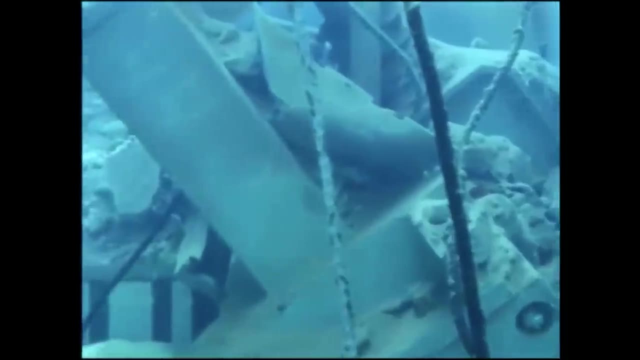 is what blocks the radiation. so without water, the radiation just goes right out into the environment. In fact, exactly that happened at Fukushima. Both the primary and backup generators failed, so the pumps and cooling systems for the spent fuel pools couldn't run, leaving the water to heat up. The situation was brought under control before enough water. 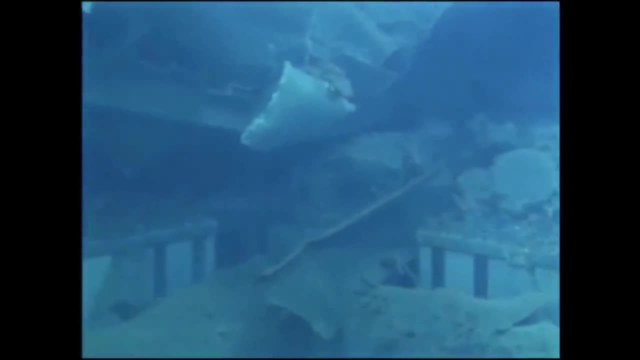 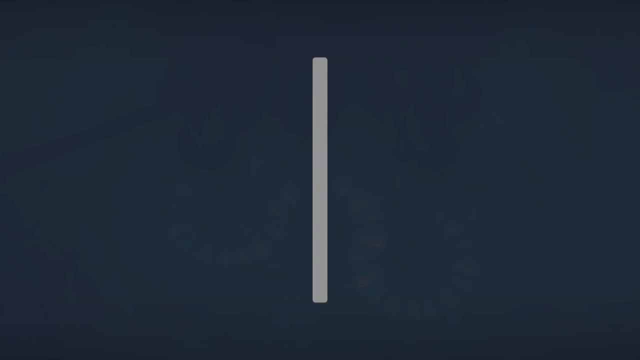 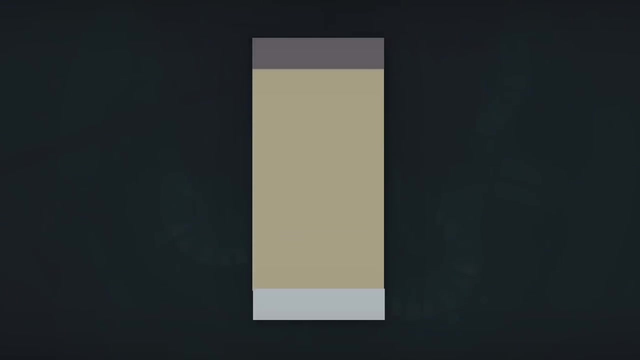 had boiled off to release significant amounts of radiation into the environment, but had it not been, thousands could have been killed. Once nuclear waste has cooled down in storage pools for ten to twenty years, it typically is encased in casks. These concrete and steel containers block in radiation, but this solution. 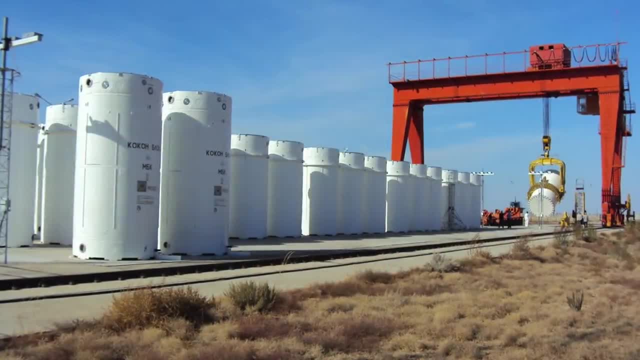 is far from permanent. It does not consider earthquakes to be an emergency, but it does to a large extent. It is not the only way to do that. It is the only way to reduce the consider earthquakes. it cannot withstand tsunamis and it would not work without humans. 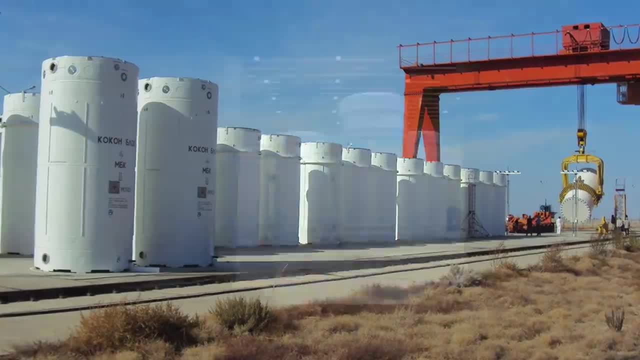 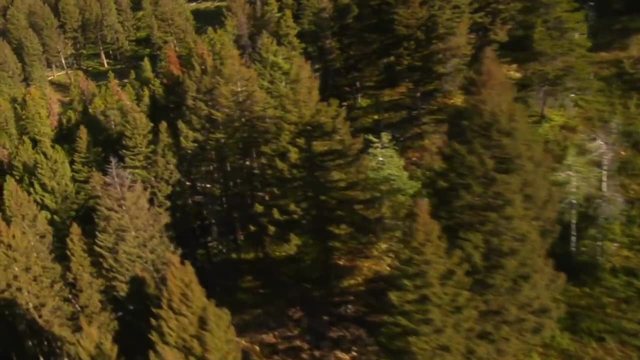 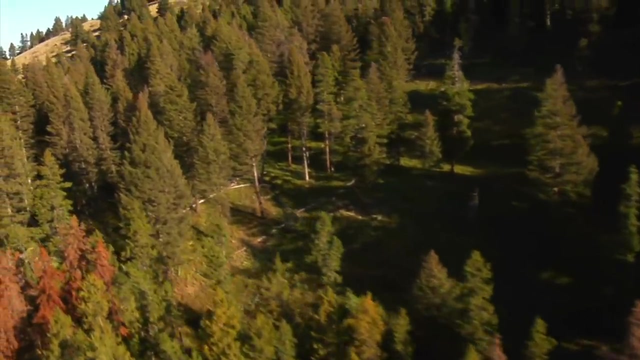 These casks require security and they require maintenance. Without humans, they could easily be damaged or breached over time and release radiation into the environment. Modern humans have only existed for about 200,000 years, so one can hardly be sure that the species will survive for the millions of years that the toxic nuclear waste will. 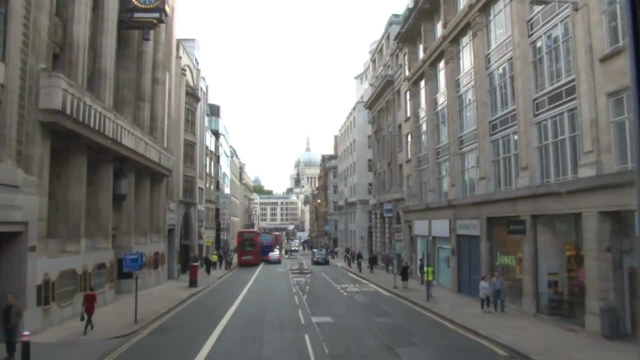 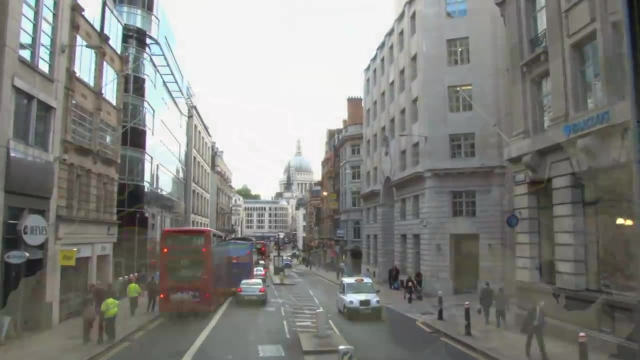 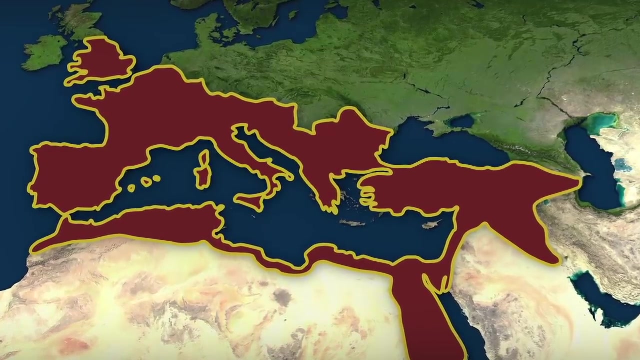 continue to emit radiation. What's more, one can hardly expect that the dominant civilizations that have nuclear technology today will continue to exist for even thousands of years. The Roman Empire was once, without a doubt, the most powerful civilization on earth. Scholars even believe that it is the most powerful civilization to have ever existed. 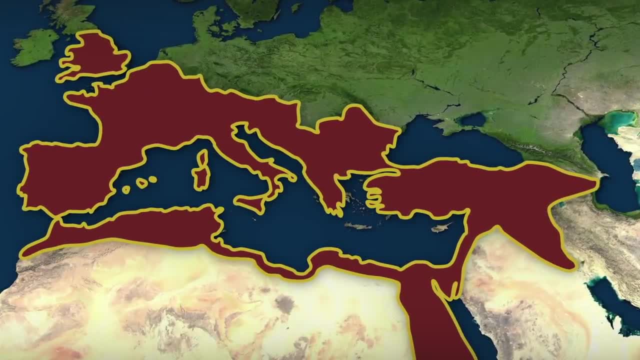 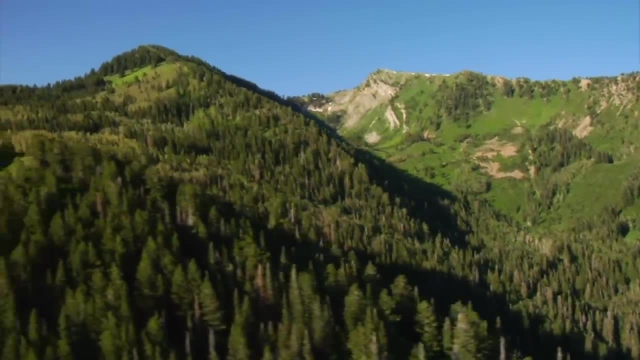 on earth—more powerful than the US, than Europe, than any modern civilization- But it fell, and so too will the West. Therefore, long-term nuclear waste storage needs to last longer. It needs to last longer than any political structure. it needs to work without the supervision. 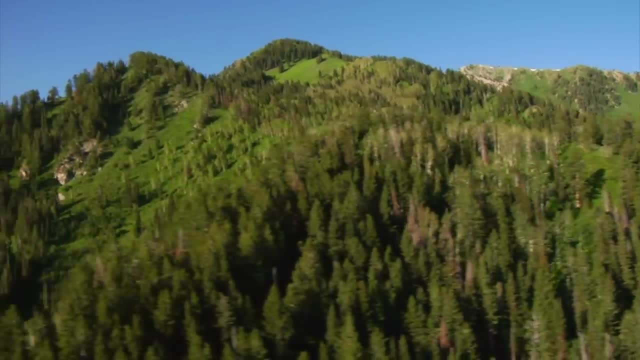 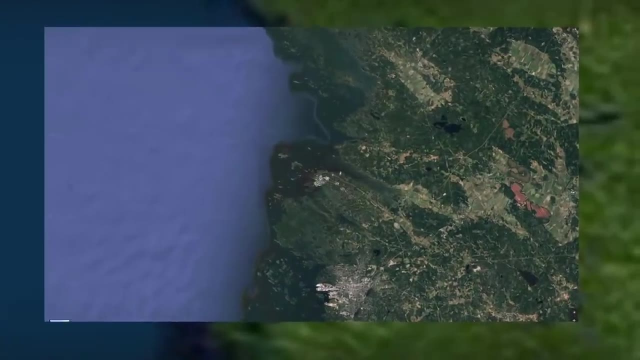 of humans. it needs to be truly and unequivocally permanent. Finland is building just that. This region is largely devoid of natural disasters. It doesn't have earthquakes, it doesn't see tsunamis, it really doesn't encounter. 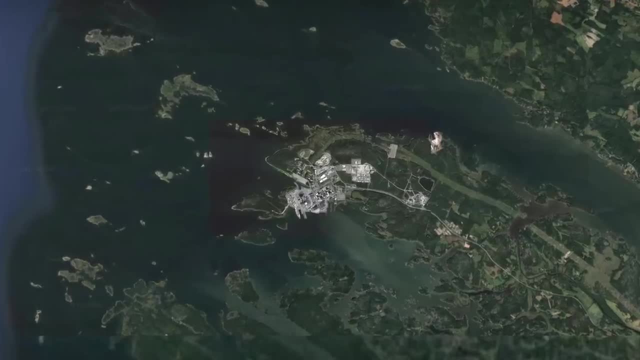 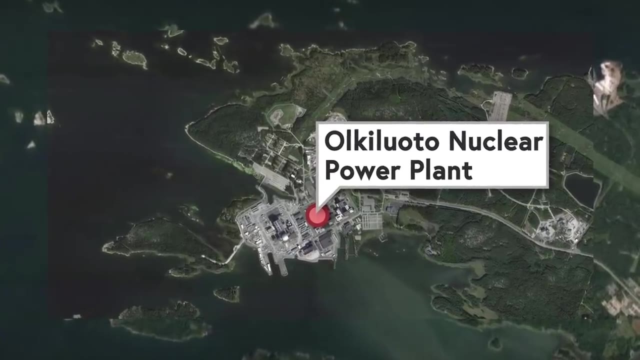 any natural phenomenon that could damage a nuclear waste storage site, especially if it's 1500 feet underground Beneath an island on the Finnish Baltic Sea coast. the country is digging—they're building the very first permanent nuclear waste storage facility in the world in this stable bedrock. 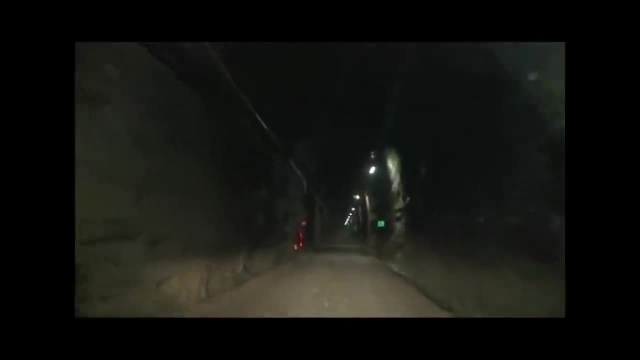 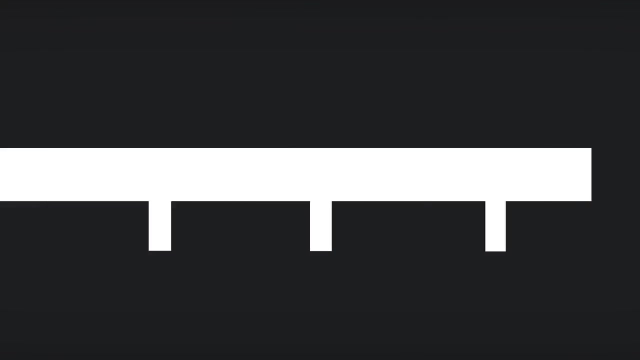 1500 feet below. Currently, they're just finishing their dig down. then very soon- in 2020, they'll start filling the facility with nuclear waste. They'll dig long tunnels with small holes in which they'll place casks of nuclear. 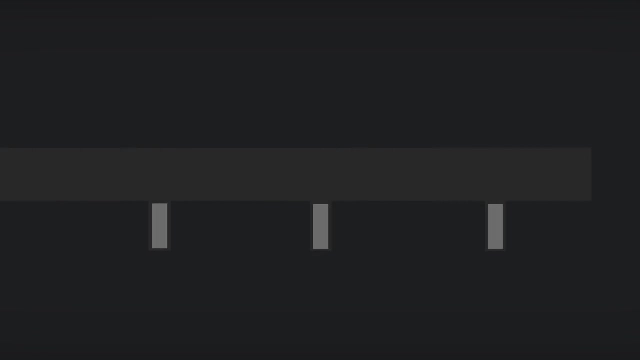 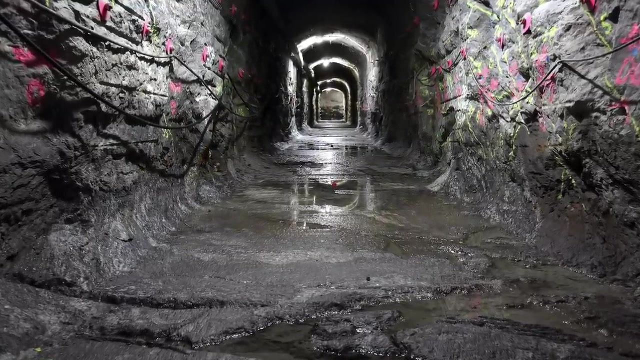 waste, then backfill the tunnels with clay to be left for an eternity. With this system, there's near-zero risk of nuclear material leaking out into the groundwater, and once it's filled in the year 2120, it can be just left for eternity. 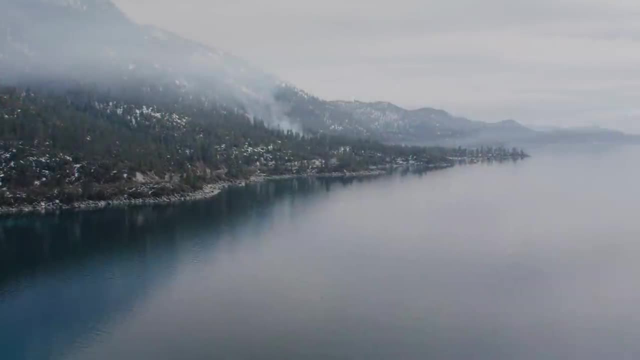 There's a risk of nuclear material leaking out into the groundwater and once it's filled, in the year 2120, it can just be left for an eternity, left forever, Because the material will be so far down and so difficult to get to no human management. 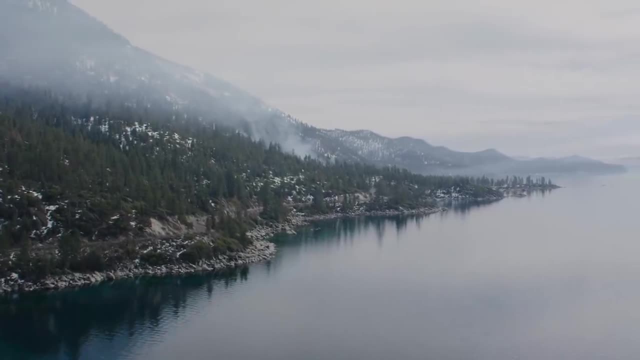 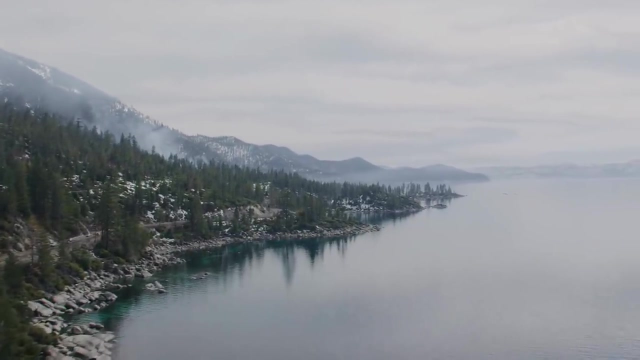 will be necessary once completed. No security, no maintenance, nothing which means it should be truly secure. but before leaving it, they do need to fight against one thing—human nature As curious beings. it's hard to combat a person's urge of discovery. 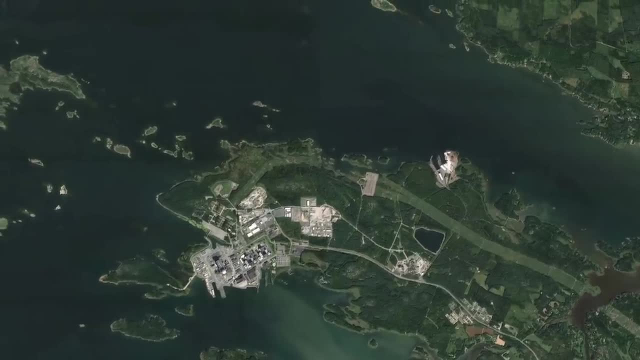 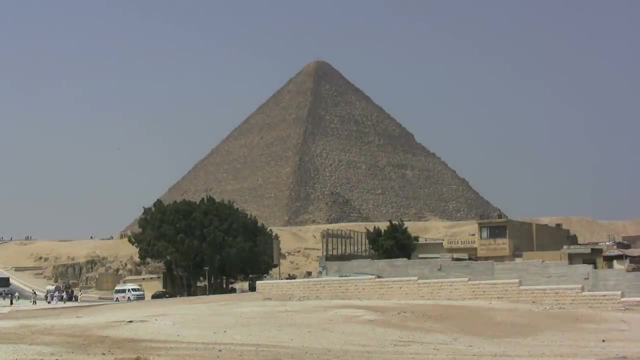 If someone finds a mysterious structure from thousands of years ago, it'd just be natural to want to open it up, and that's a problem for nuclear waste sites. We essentially did just that with the pyramids in Egypt. These structures were built as the final permanent resting places for the elites of 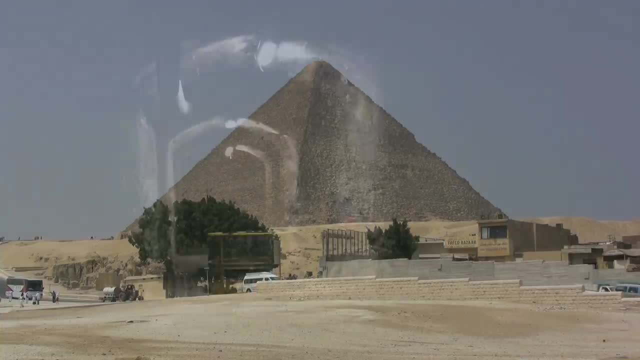 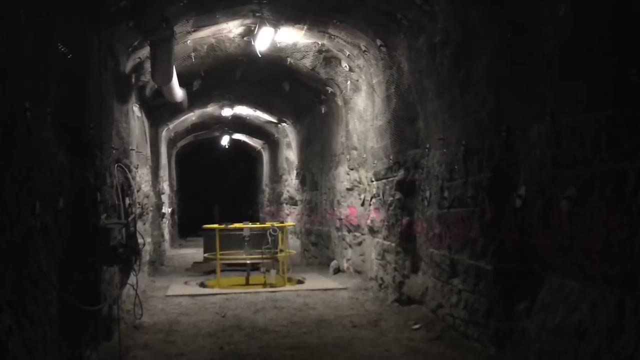 Egypt, and we opened them up because we were curious. Opening the nuclear storage facilities would release radiation into a future civilization, so we have to tell them to leave the sites alone. but that's easier said than done. The US Department of Energy commissioned a study on how to communicate the danger into 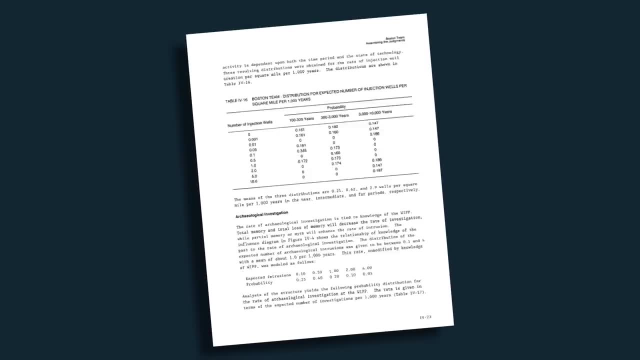 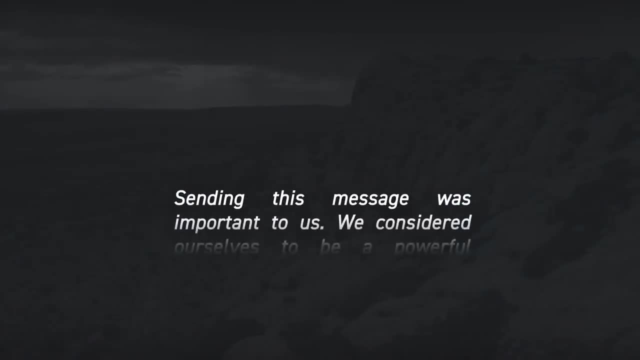 the far future. The key is to create a message that conveys how uninteresting, how unimportant and how dangerous nuclear waste is. They settled on the following text: Sending this message was important to us. We considered ourselves to be a powerful culture. 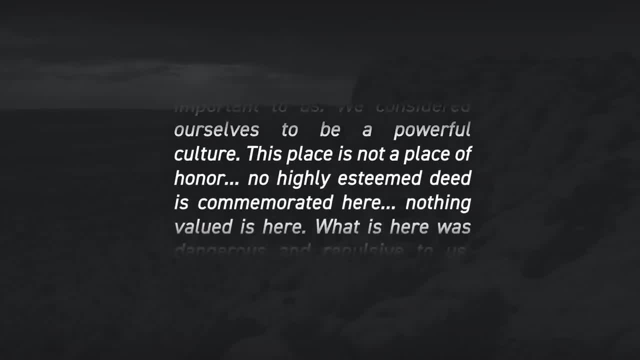 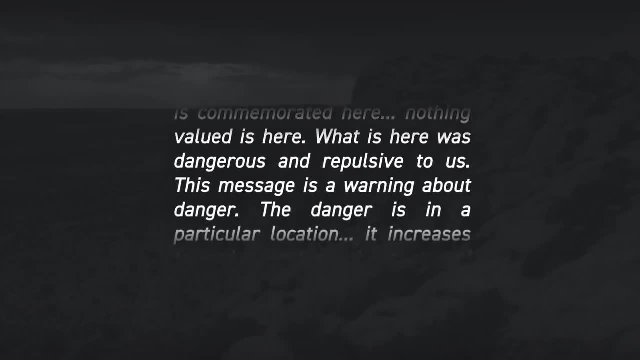 This place is not a place of honor. No highly esteemed deed is commemorated here. Nothing valued is here. What is here was dangerous and repulsive to us. This message is a warning about danger. The danger is in a particular location. It increases towards the center. 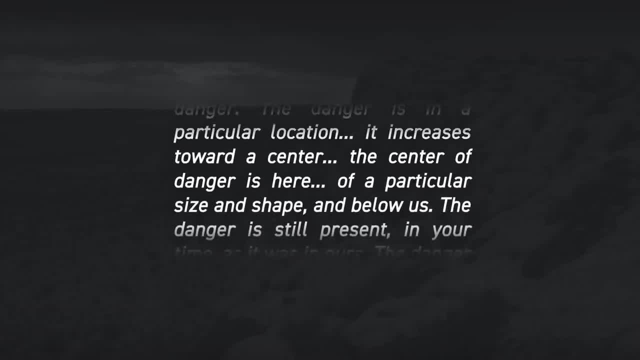 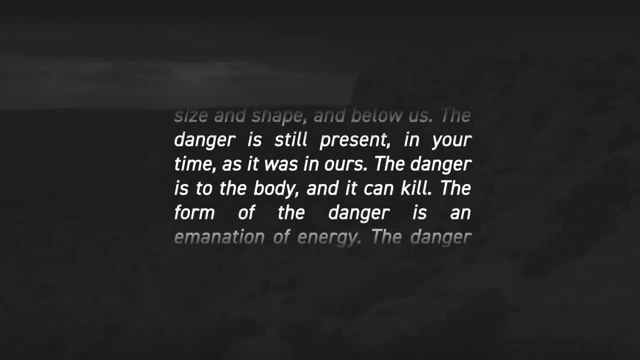 The center of danger is here, of a particular size and shape, and below us. The danger is still present in your time as it was in ours. The danger is to the body and it can kill. The form of the danger is an emanation of energy. 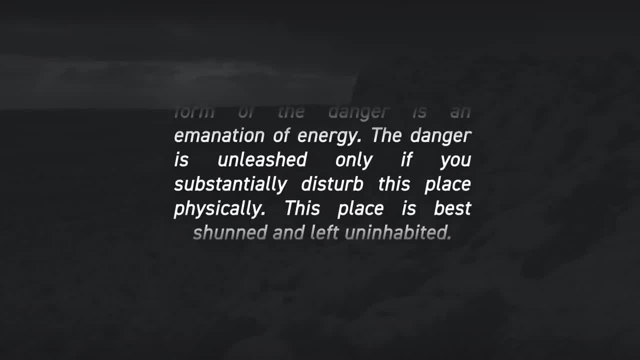 The danger is unleashed only if you substantially disturb this place physically. This place is best shunned and left uninhabited. The idea would be to translate a message like this into every United Nations language—Arabic, Chinese, English, French, Russian and Spanish. 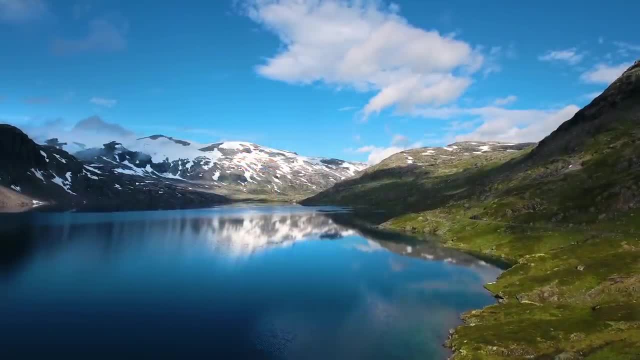 The idea would be to translate a message like this into every United Nations language—Arabic, Chinese, French, Russian and Spanish. There's a reasonable hope that, at least in the next couple thousand years, one of those languages would be understood. 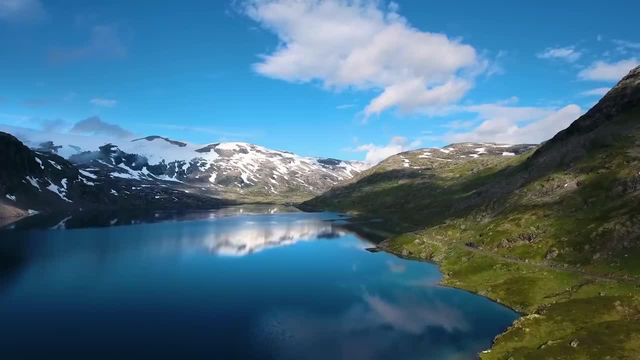 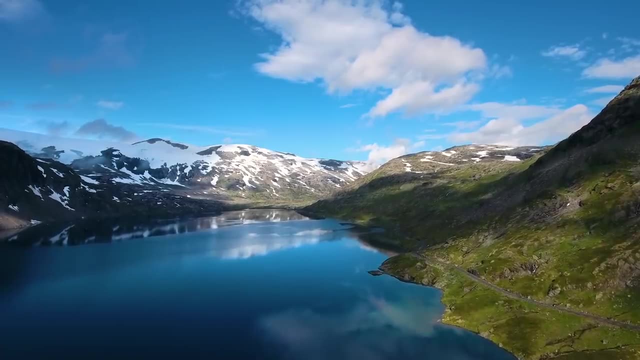 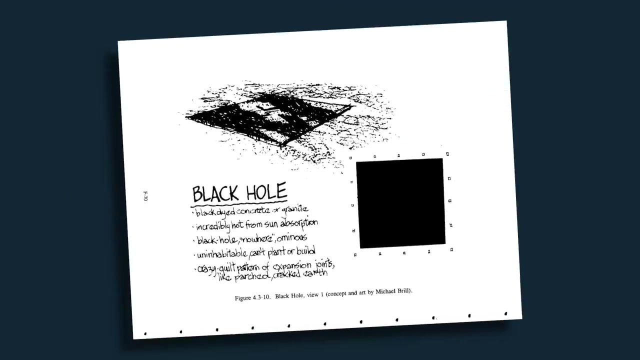 But in the scope of hundreds of thousands of years, there's just little expectation that these languages would survive. There's not even a reasonable expectation that humans will survive. So you need to convey the same message without language. What the study suggests is to further push the message by building a landscape that conveys. 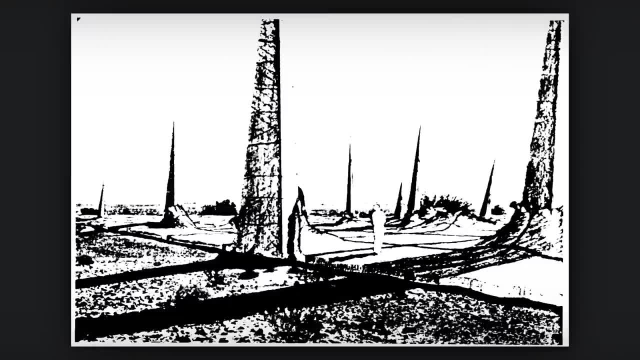 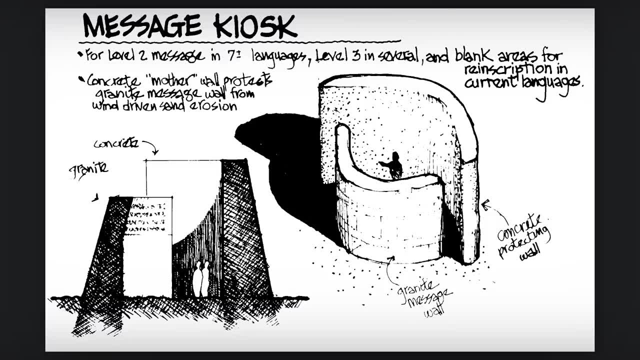 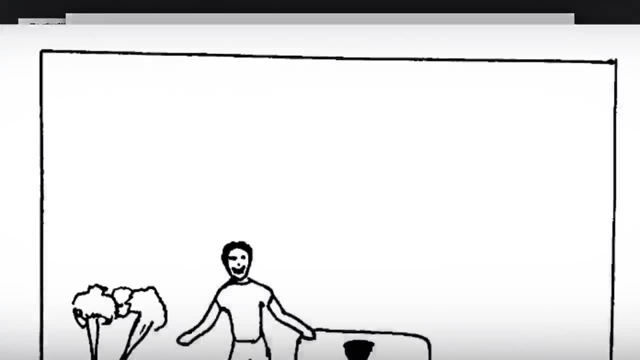 danger. To satiate the discoverer's curiosity, it's also suggested to add monoliths explaining the history of the site through pictographs. Also included would be images like this engraved in stone, conveying that the substance has danger that would be passed onto humans if touched. but the difficulty of this is that 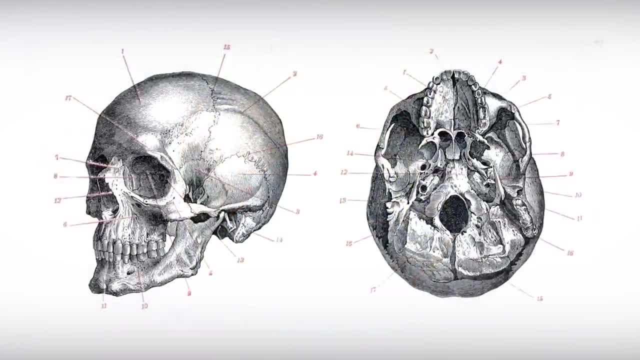 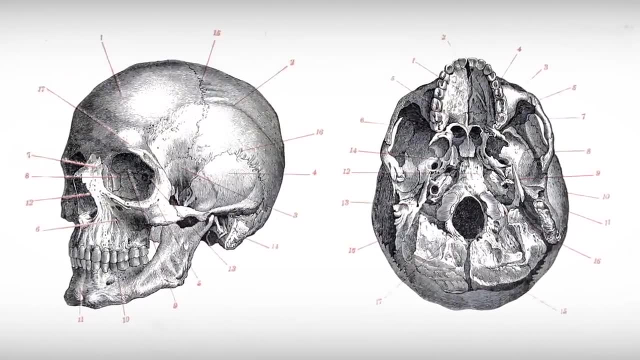 it very well might not be humans exploring Earth 100,000 years from now. It could be a species that doesn't recognize the likeness of what might be a long-extinct species. What some have suggested is to just let the site be forgotten, to not mark it at all. 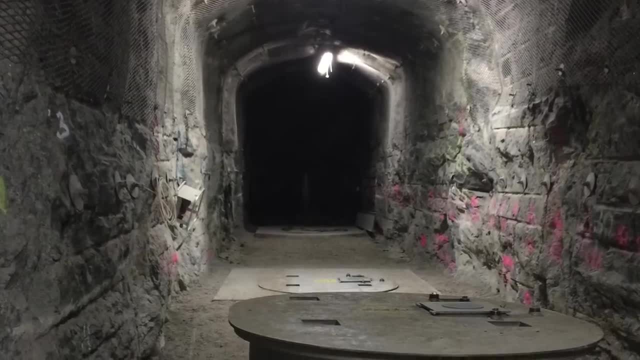 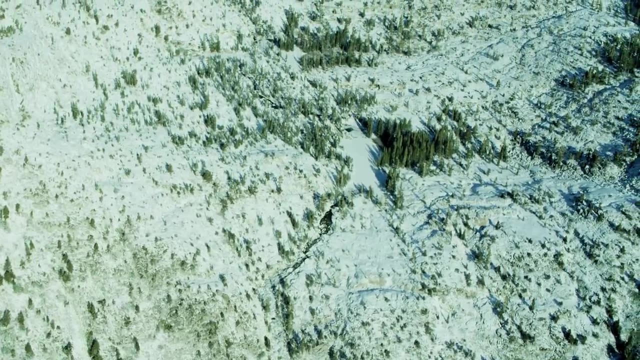 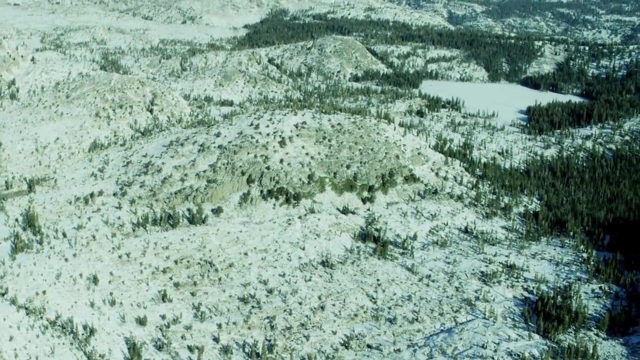 to just seal it up and leave, but having something that significant disappear isn't simple. The site in Finland is designed to not need security or oversight, but its current location is very well documented in a potentially irreversible way, With books and brains, and the internet records of the site might exist until at least the